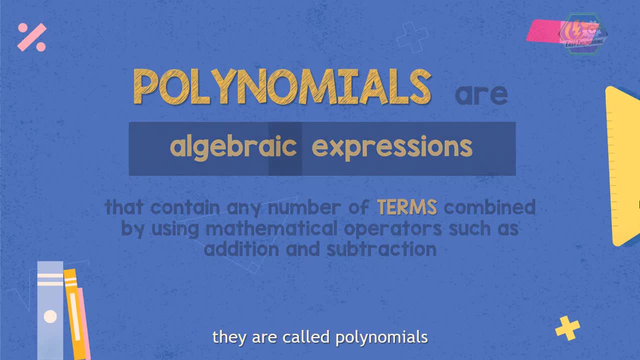 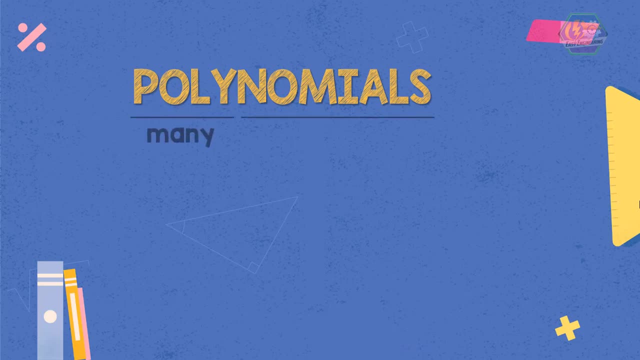 three terms or more terms. they are called polynomials. Polynomials also come from the word poly, which means many, and nomial, which means terms. These are some examples of polynomials. Polynomials also have different names based on the number of terms. 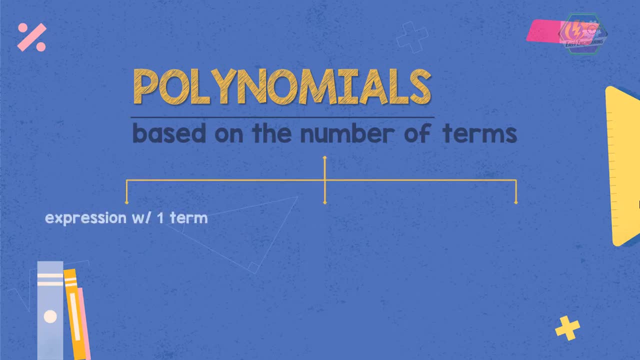 So if you have an expression with one term, it is called monomial. If you have an expression with two terms, it is called binomial, And an expression with three terms is called trinomial. If we have an expression 4x, this is called a monomial. Even a whole number like number 3,. 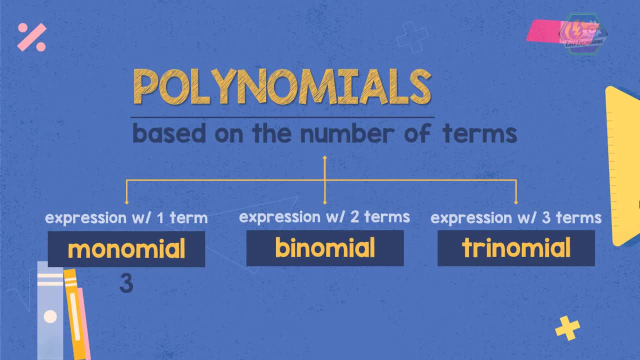 for example, is called monomial 1. gray pack is an expression of trinomial 2. white pack includes three terms. which is, bydio, been Soldier today's distinction? Yeah, I'm sure you'd know why. It's because we shaking a box. 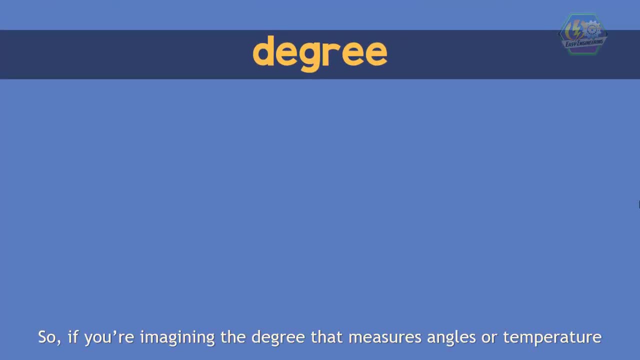 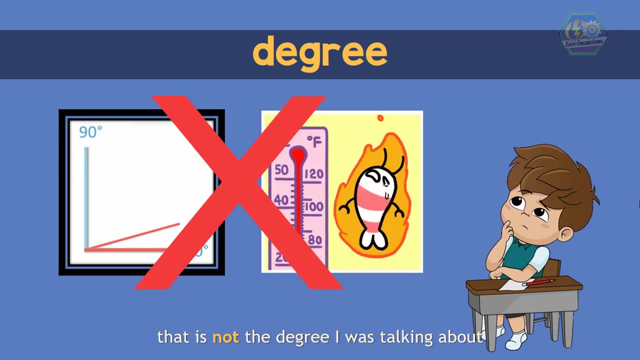 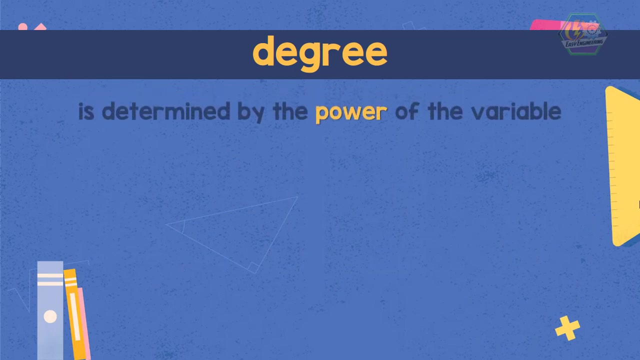 call the degree. so if you're imagining the degree which measures angles or temperature, I'm sorry to disappoint you, but that's not the degree I was talking about. degree of a term is determined by the power of the variable. so if you have a term x squared, then we can say that the degree of the term is 2 or it is a. 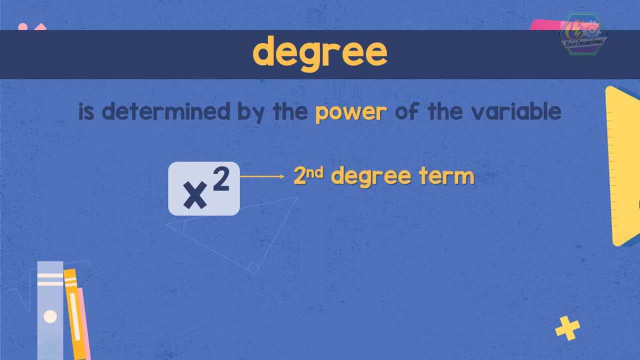 second-degree term, or we have a term 9x cubed. the power of the variable is 3, so it is a third-degree term. what if we have a term with more than one variable? how can we determine the degree of the term? good question right now. if we have 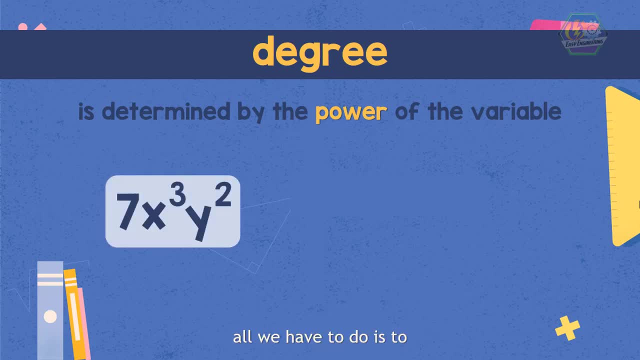 a term like this, all we have to do is to add up all the powers of each variable to get the degree of that term. so in this case, the variables has a power of 3 and 2. therefore, it has a degree of 3 plus 2, which is 5 or fifth degree term. 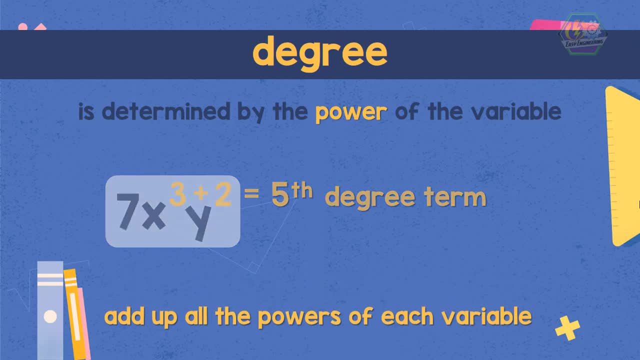 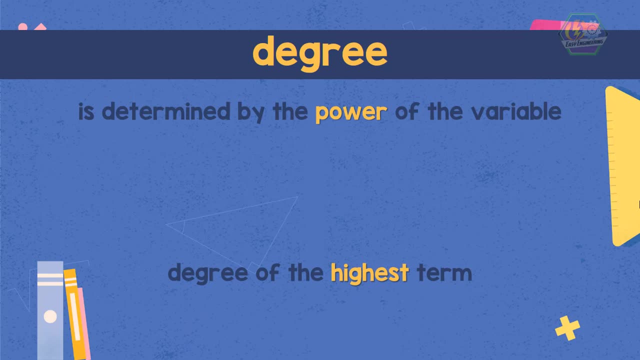 and now it's with the polynomials. so in polynomials we need to determine the degree of the highest term. if we have a polynomial 7x cube plus x squared word minus 5, then this polynomial is a third degree polynomial, since the highest degree. 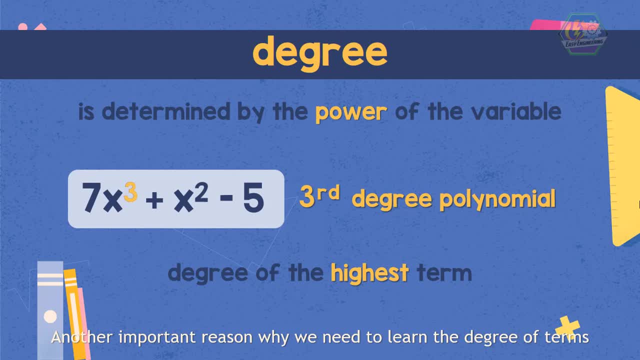 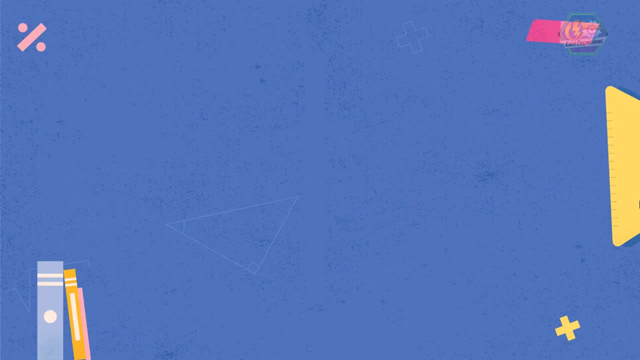 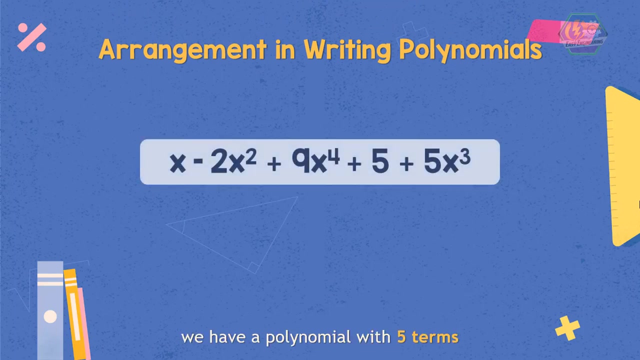 term has a power of 3.. Another important reason why we need to learn the degree of terms is because it helps us to decide the arrangement. in writing. polynomials: For example, we have a polynomial with 5 terms. All we have to do is rearrange the terms from highest degree to lowest. 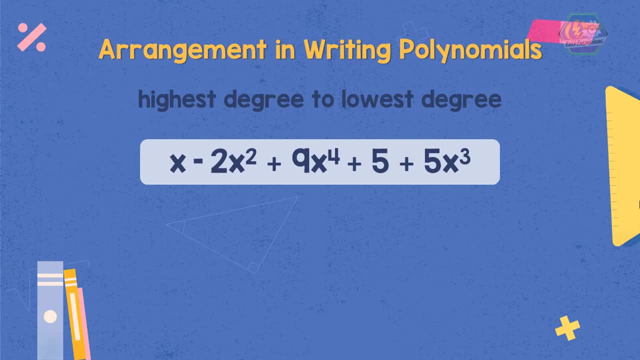 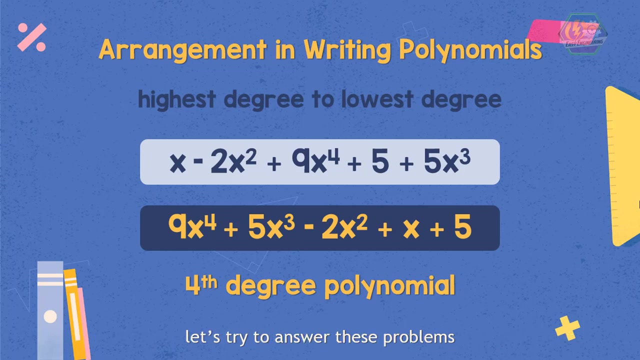 So for this example, we'll become 9x to the power, 4 plus 5x, cube minus 2x, squared plus x plus 5, and this example is a fourth degree polynomial. So now that you already learned what polynomials are all about, let's try to answer. 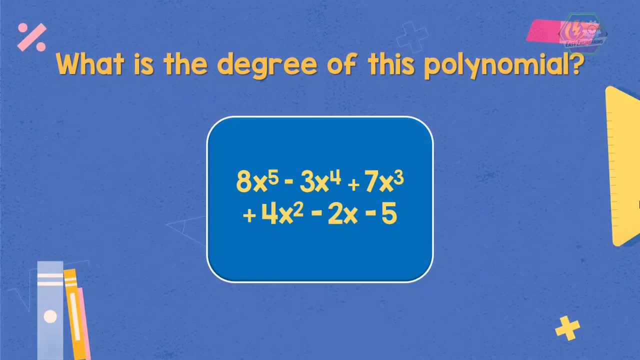 these problems. So what is the degree of this polynomial? 8x to the power 5 minus 3x to the power 4 plus 7x, cube plus 4x, squared minus 2x minus 5.. Correct, This is correct. 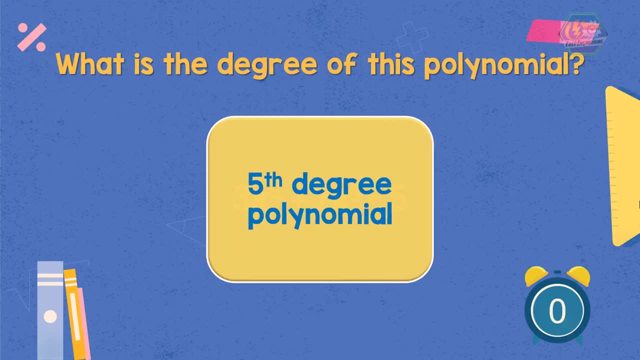 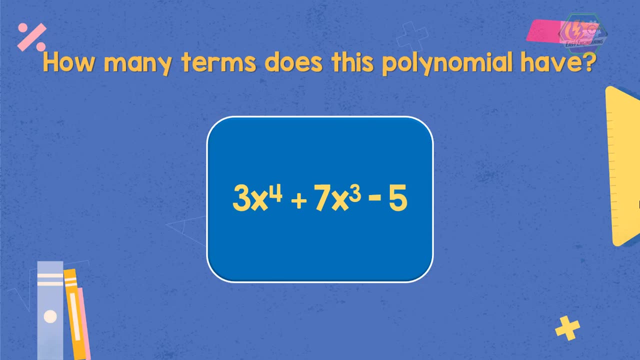 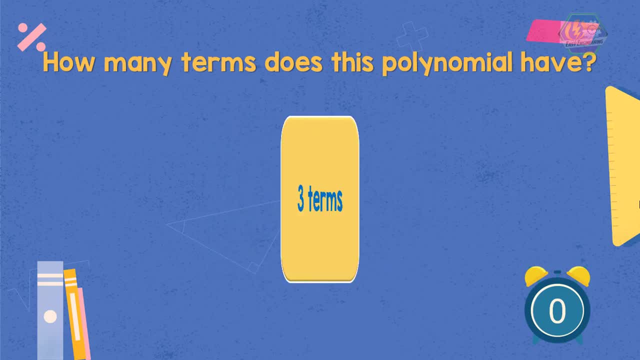 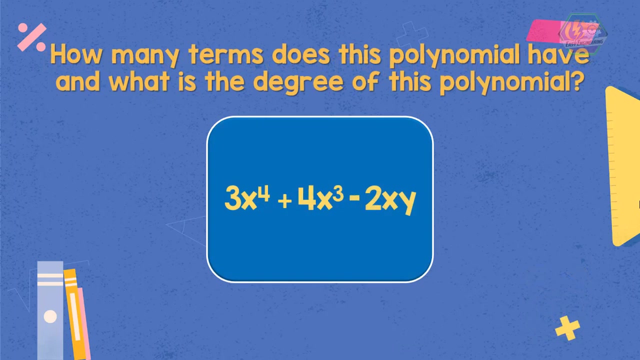 3x squared minus 7x squared minus 7.. That's right. This polynomial has 3 terms. Notice that the question is asking how many terms, not the degree of terms, So we need to be careful in reading the problem. Now for the last problem.